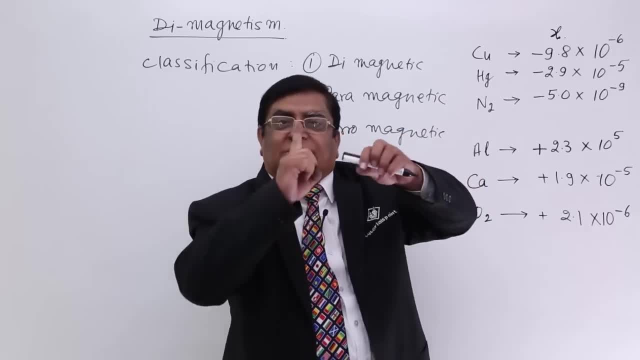 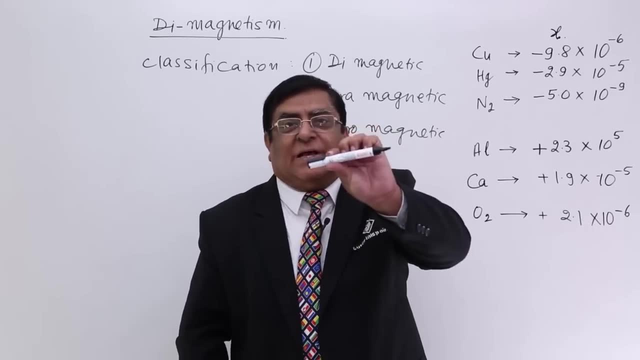 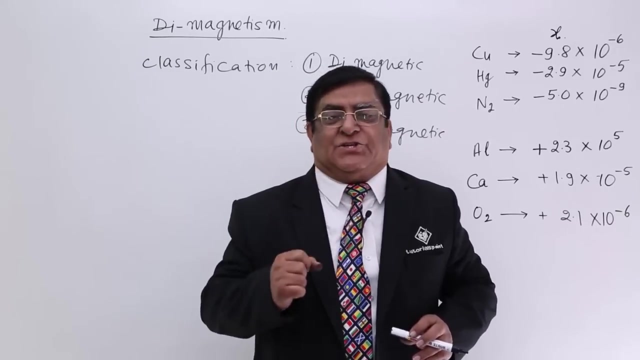 field in this is 80.. Why 80?? Because this has produced a opposite magnetic field in this equal to 20.. Such material are known as Dimagnetic. Sometimes it is said that magnetic fields will have multidimagnetic nature. Then Gauss gave a definition of magnetic field In the case of 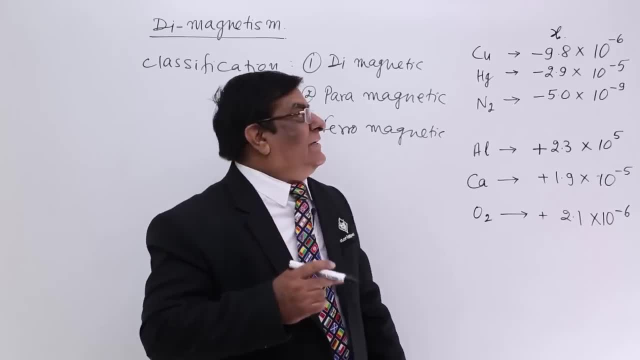 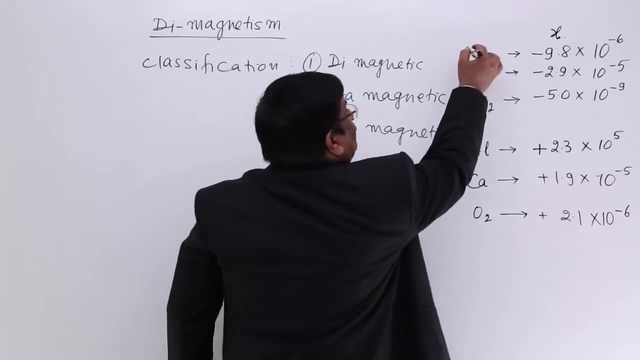 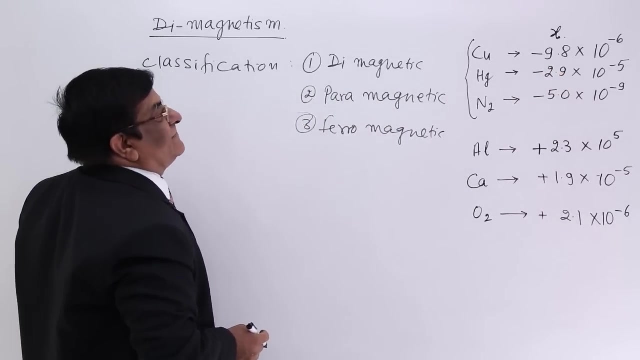 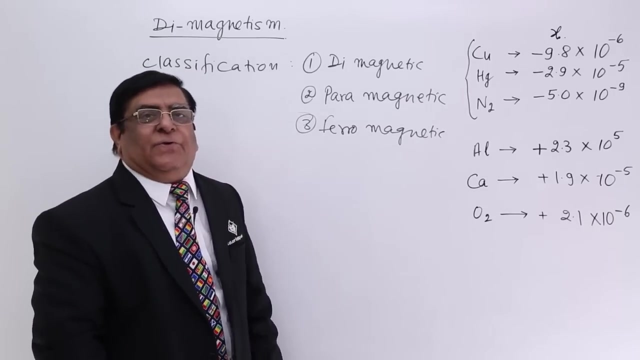 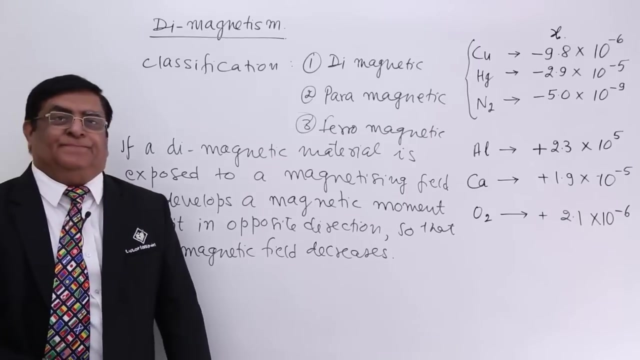 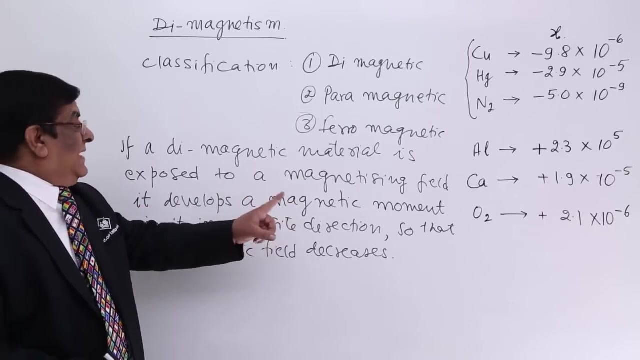 magnetic fields, it is called magnetic field, The magnetic fieldочки. can happen that magnetic field rating works fine. Okay, characteristics, and we will study those characteristics. So first we will write what is diamagnetic material. If a diamagnetic material is exposed to a magnetizing field, it develops a magnetic 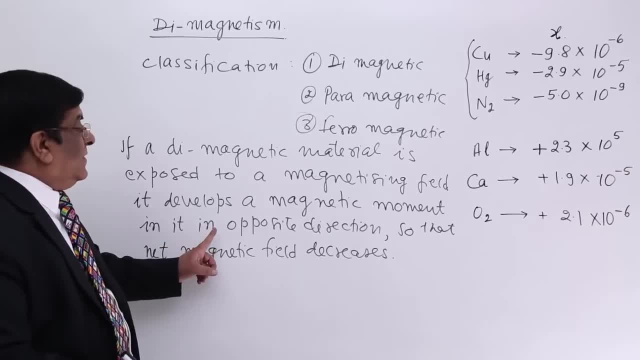 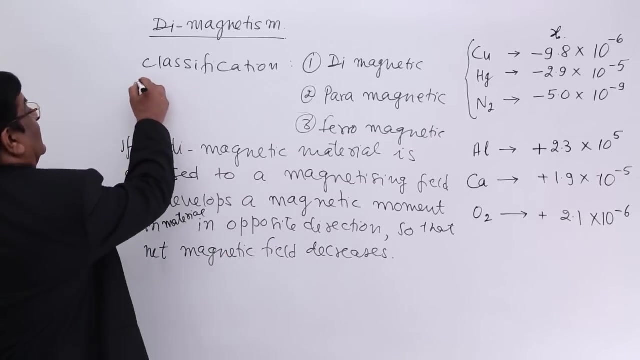 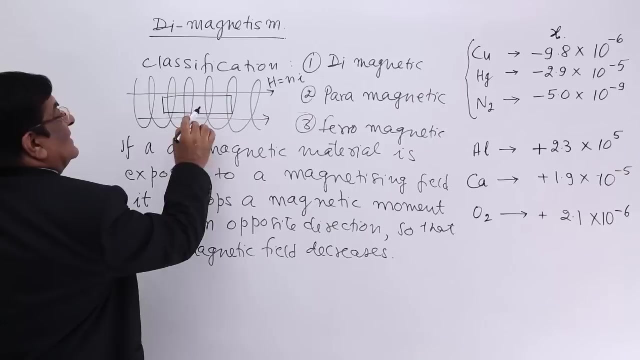 moment in it in opposite direction. In it means in material in opposite direction, so that net magnetic field decrease. Here the magnetic field developed in this direction due to current H is equal to 0. Then I put a diamagnetic material here. In the diamagnetic material, the magnetic field. 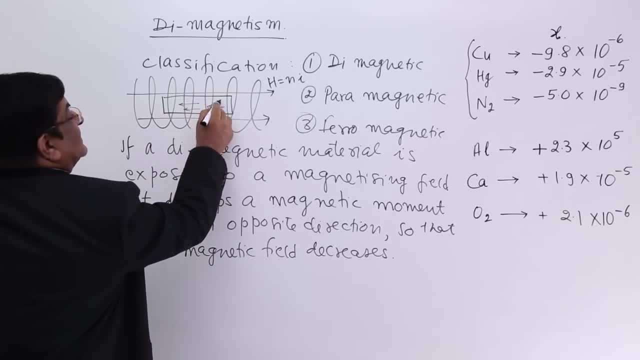 is developed in this direction. This is induced magnetic field, This is Bm magnetic field. in the material. This is B, which is equal to mu 0 H B. mu 0 H is in this direction, while Bm. So what will be the net B? Net B will be B0 plus Bm, which is in opposite direction. 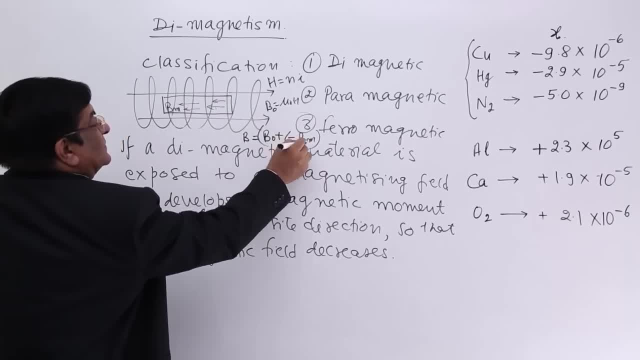 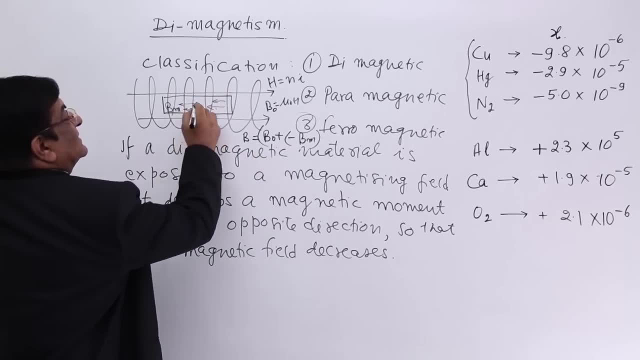 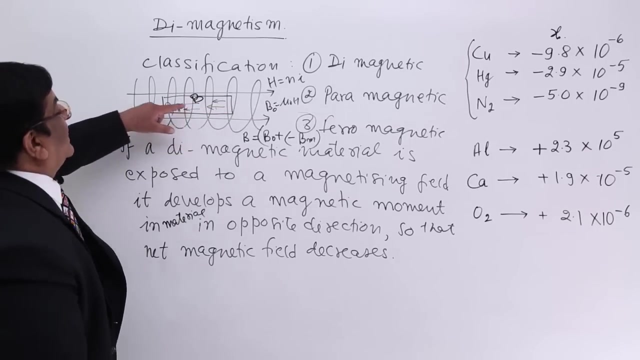 So this is minus Bm, So this value will decrease inside this. So inside this, the net magnetic field is how much B? Bm is what magnetization developed in the material- This is B0- by this magnetic field in this direction. 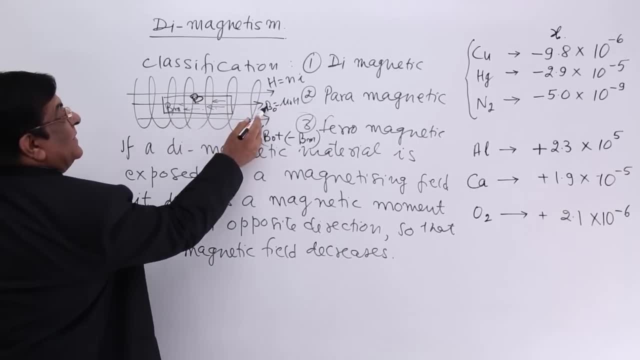 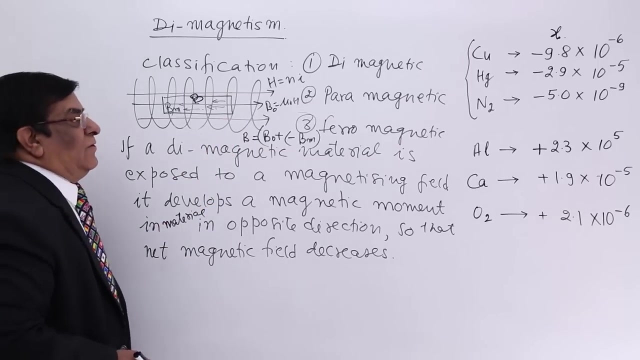 So how much is the total here? How much is the net here? B0 applied by the current minus. this developed in the magnetic field, developed in the material which is in opposite direction. Such material is known as diamagnetic material. Now there are certain other features of diamagnetic. 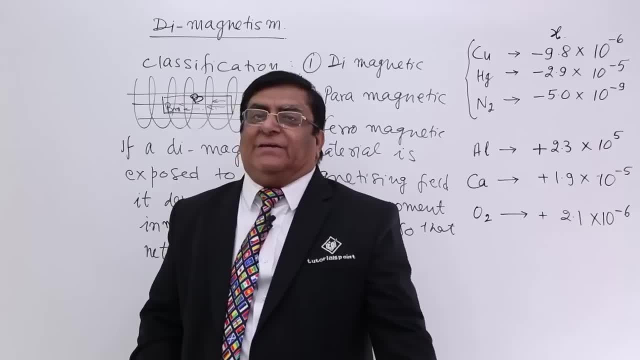 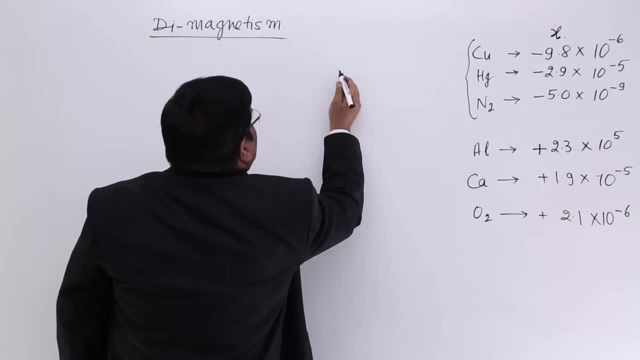 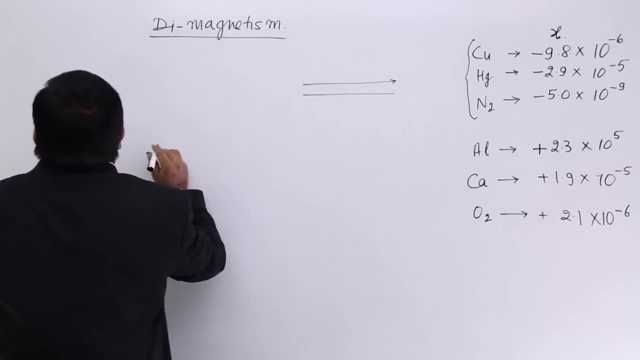 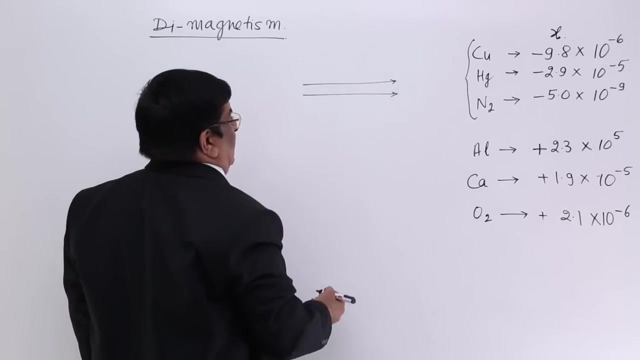 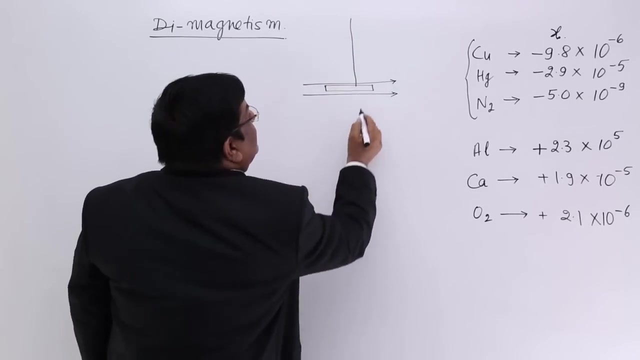 material like this does not like magnetic field. It is expressed by a few experiments. One of this example is: yes, here we have magnetic field. If I put a rod of this diamagnetic material and I place it in this direction By a thread, then what I see? that it automatically turns this way and goes out. try to go out. 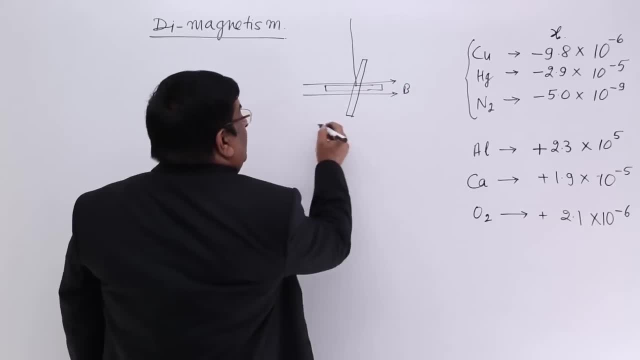 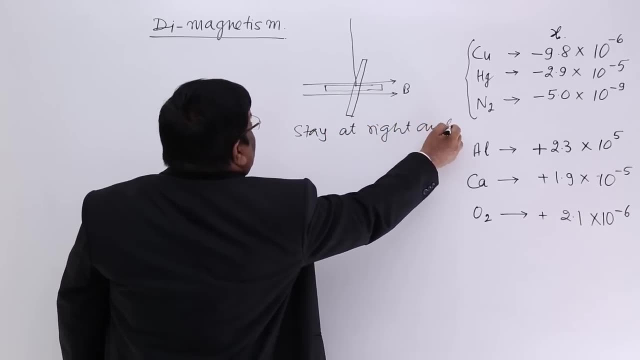 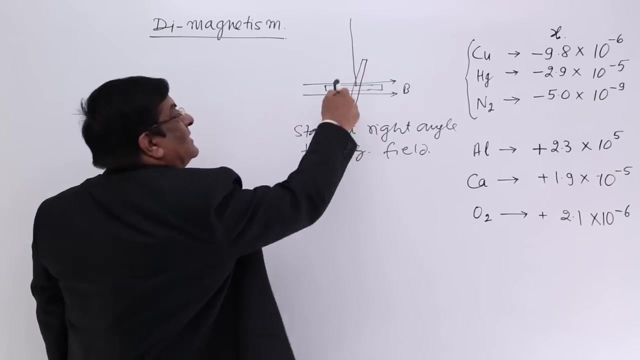 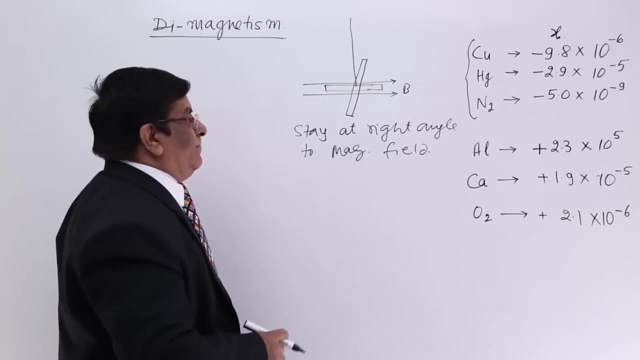 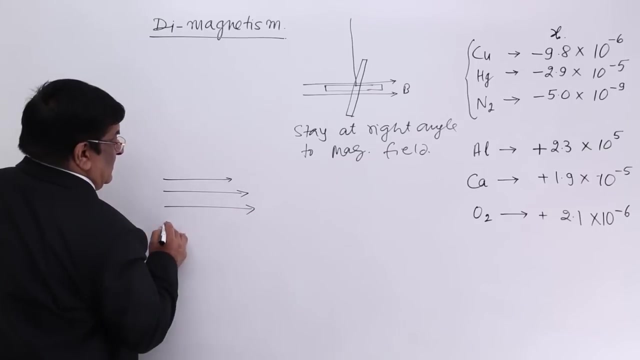 from this magnetic field. So it always stay at right angle to magnetic field, to external magnetic field, because this does not like magnetic field And it wants minimum exposure to the magnetic field, ok. Other thing: if there is a magnetic field here and I am putting a diamagnetic material here- 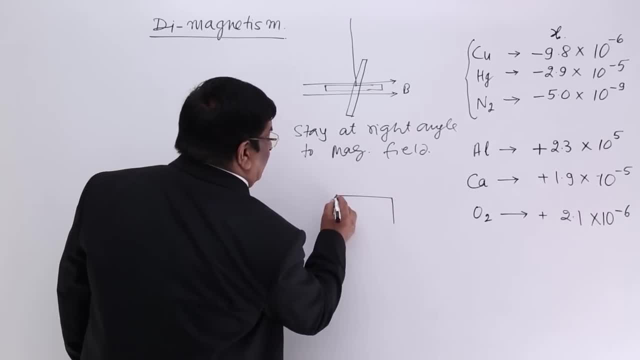 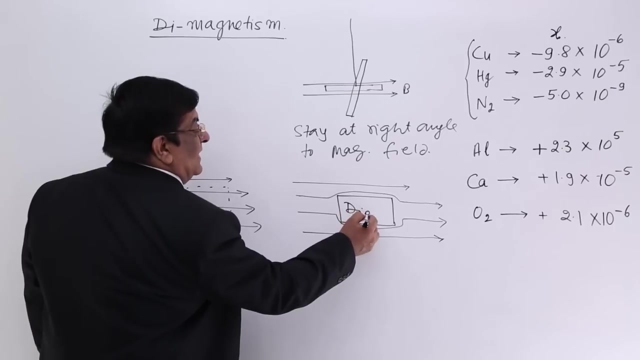 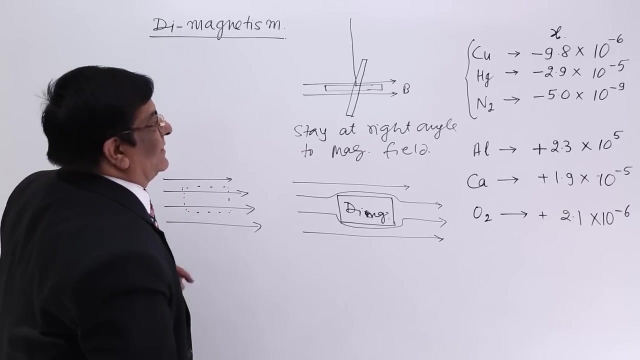 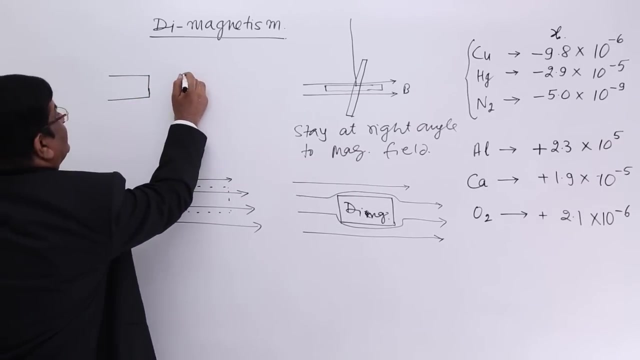 what will happen? Answer is: this is diamagnetic material, and these four these will be like this, This: it will not allow magnetic field to pass through it because this is diamagnetic, So such material is known as diamagnetic. See, once again, we have two magnets here north. 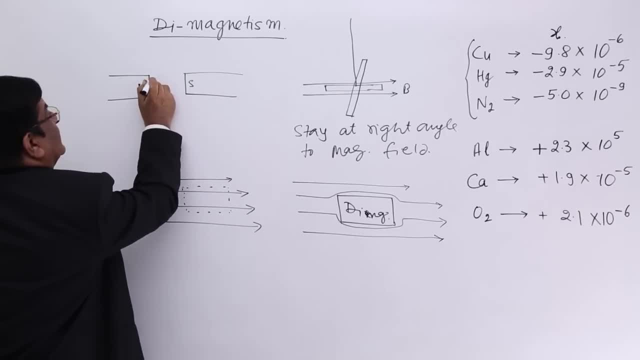 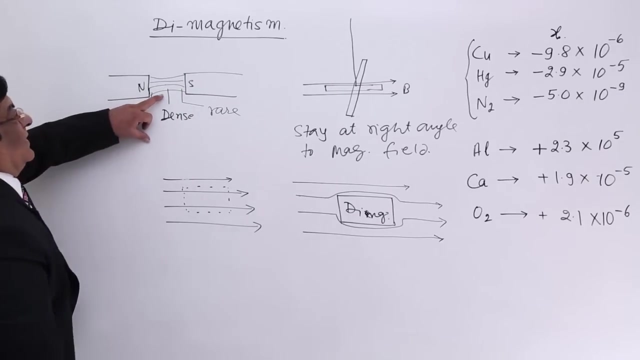 south. They are very close to each other and here we have a magnetic field and that magnetic field, because of these two, is like this: Here it is magnetic field is dense, and here it is rare, because of this pole and this pole both join here. Here it becomes denser, magnetic field is stronger and here it is rarer. 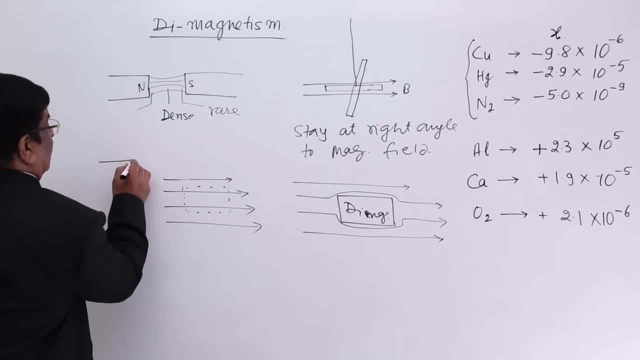 If I increase the distance, if I increase the distance like this, north and south, then this will go like this and for this, here it is rarer and at the corners it is denser Magnetic field because of these two. ok, Now what do we do? I put a diamagnetic material here and I put 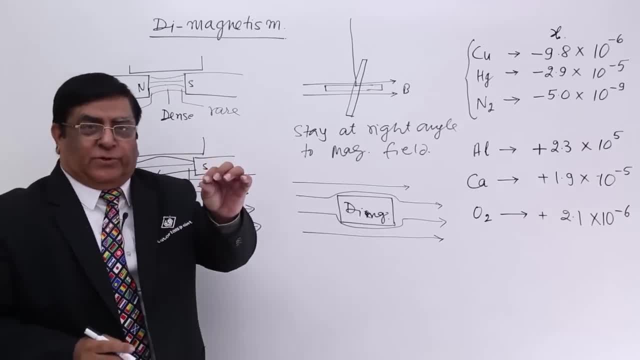 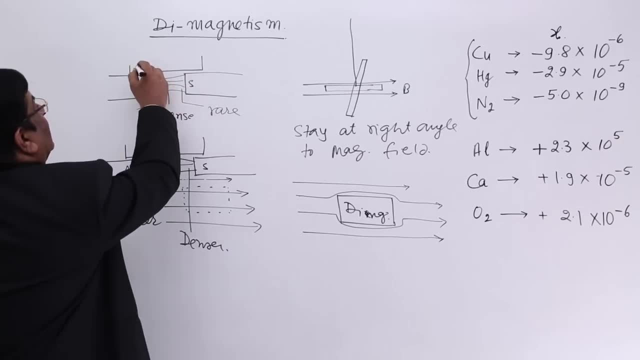 the same diamagnetic material, here in the form of powder, and then I tap it. When I tap the powder here, diamagnetic material makes a bundle like this: It is denser here. Wherever it is denser, this material will be less, and where it is rarer, here magnetic field is. 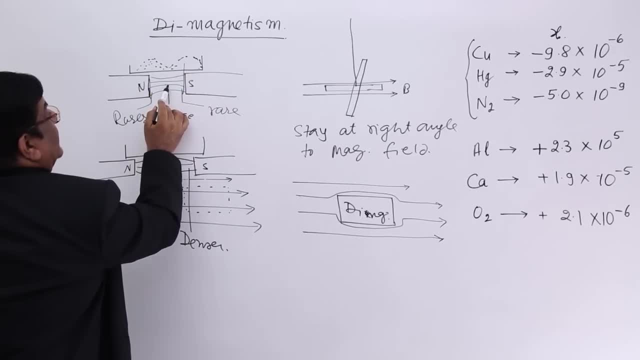 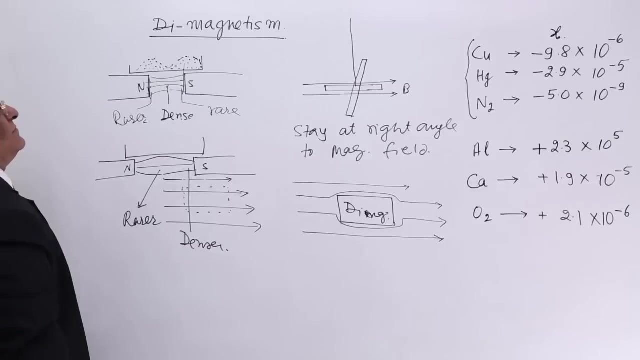 weak compared to this point. Here. magnetic field is 50, here it is 50,, here it is 75. So at place of 75, it will not like to come, At the place of 50, it has to come because 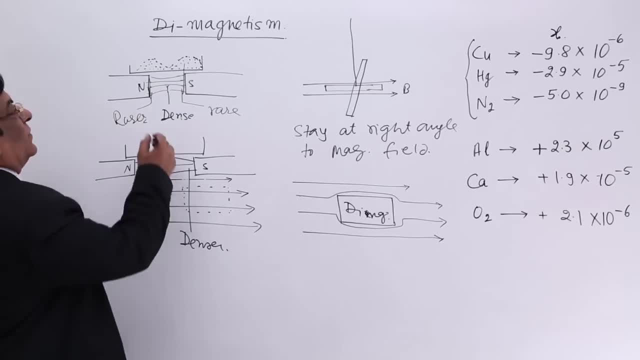 50 is less than 75. So this has to be done. This happens when they are very close to each other, very close, But if we take them away, then magnetic field are like this and this becomes rarer. and these corners now again. 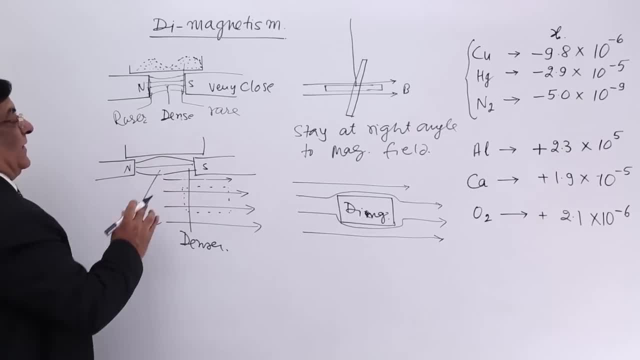 these are 50,, 50, but this has become 40. Now what we find? that the same material. when we tap it here, this material gather like this This way. So what does it mean? That dielectric material would like to remain at the place.